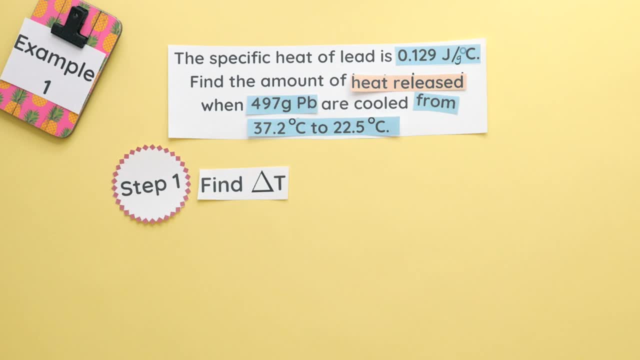 we will start with step one, which is finding our change in temperature. Our change in temperature is our final temperature minus our initial temperature. When we do this, we get negative 14.7 degrees Celsius as our change in temperature. Step two: Plug everything into the formula. 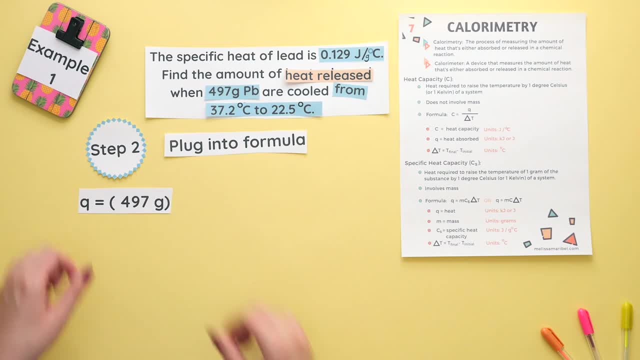 Here's the formula we will use. We have our mass in grams, specific heat capacity and change in temperature. Multiply all of these together and our units of grams in Celsius cancel out and we are left with heat in joules. Make sure to round to three sig figs. 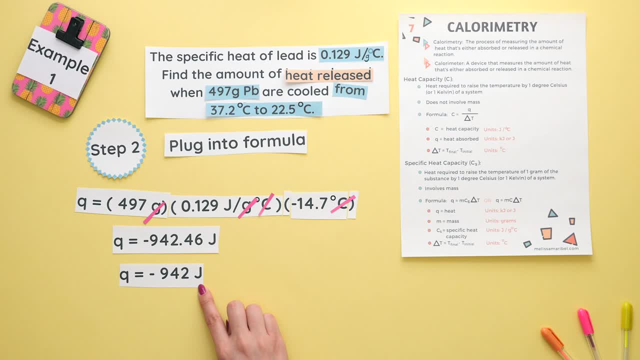 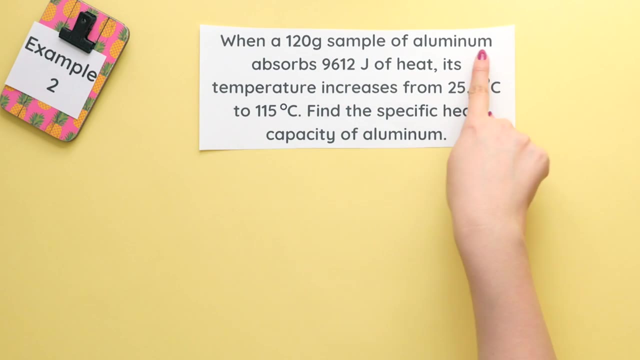 Now we could have written our answer as negative- 942 joules- or we can write it without the negative, As long as we put 942 joules are released. Both answers are correct here. Example two: When 120 gram samples of aluminum absorbs 9611 joules of heat energy. 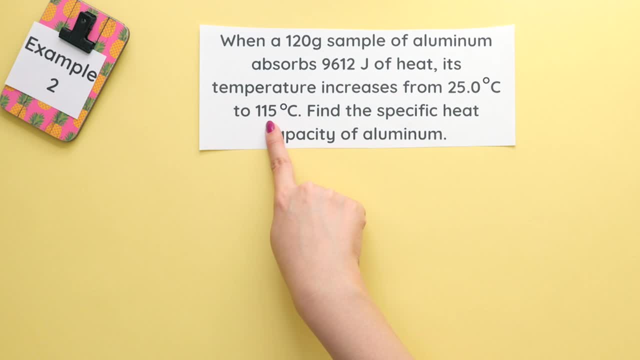 its temperature increases from 25 degrees Celsius to 115 degrees Celsius. find the specific heat capacity of aluminum. Let's identify what we are given and what we are finding. We are given the mass temperature, current cartridge output, length and location of thecedảng analyses. 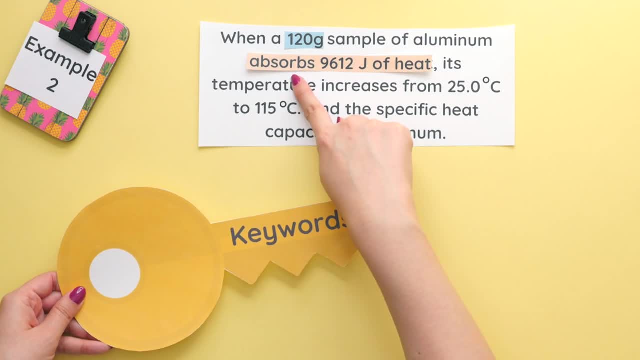 values and readings of energy. including these values, The Putty todavía Indian is shown here and we David over. We are somewhat low. You can find the Hitler configuration starting at 14.5 degrees is positive, since our keyword here is absorbs from 25 degrees Celsius means. 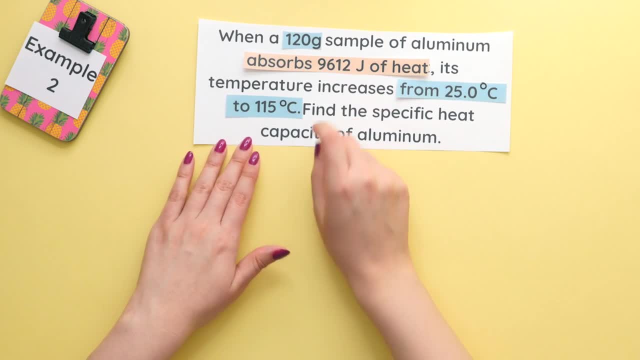 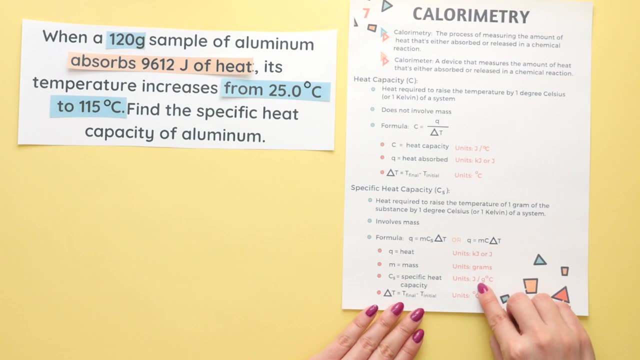 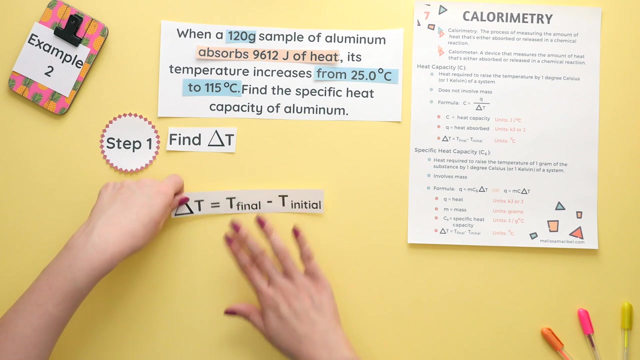 this is our initial temperature to. 115 degrees Celsius means this is our final temperature and we are finding the specific heat capacity, which has a unit of joules divided by grams Celsius. Since everything is in its proper unit, we will start with step one, which is to find our change in temperature, Final minus. 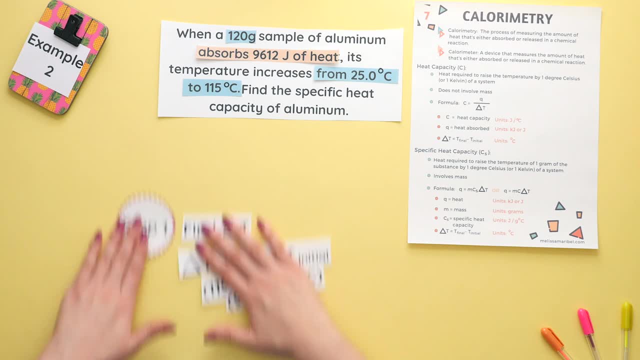 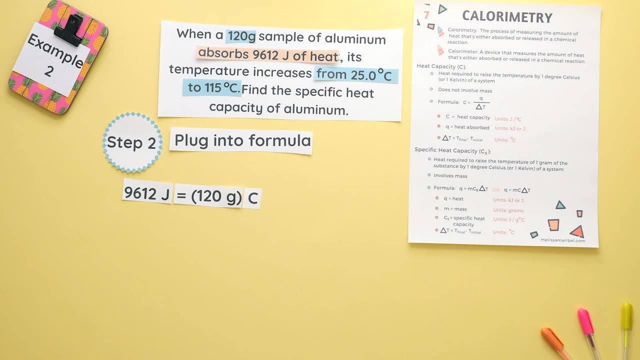 initial gives us 90 degrees Celsius. Step two: plug everything into the formula. So we know our heat, our mass, and we are looking for the specific heat capacity. and we just found our change in temperature. So multiply these two values together so we get this new value with our units of grams Celsius. Now to get 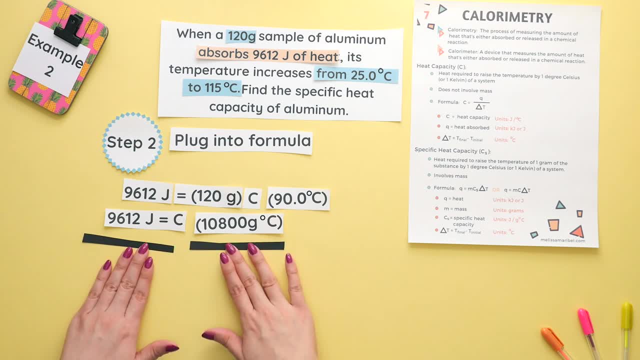 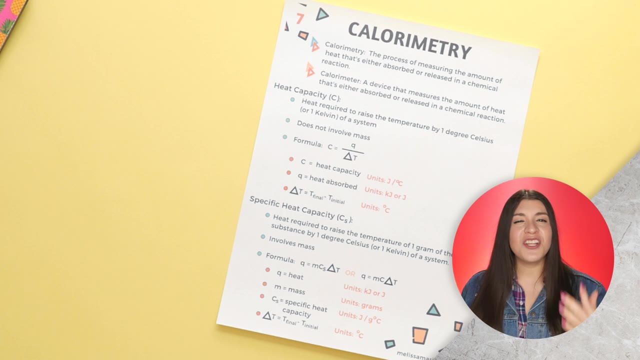 the specific heat capacity by itself. we will divide both sides by this value, and our specific heat capacity is 0.89 joules per gram Celsius. For more help with calorimetry or thermochemistry, make sure to check out my thermochemistry guide, which is right over here, I know.